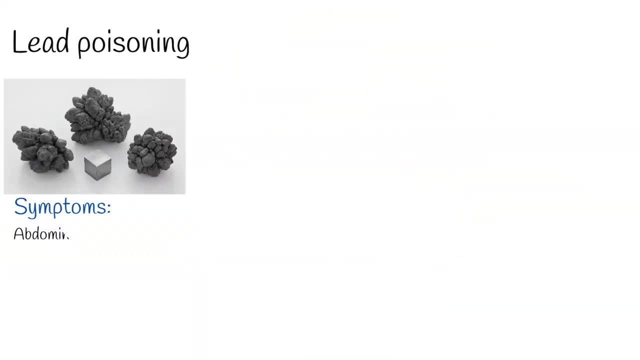 Lead poisoning. Lead poisoning symptoms include Abdominal pain, constipation, feeling tired, irritable, loss of appetite, memory loss, pain or tingling in the hands and feet. Prolonged and high levels of lead poisoning can cause. 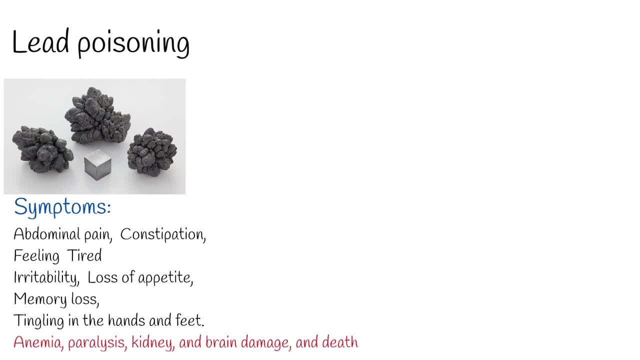 anemia and heart disease, Anemia, paralysis, kidney and brain damage and even death. Lead poisoning affects children more easily and may cause neuronal damage and intellectual disability. Lead dust and fumes have no smell, so exposure to lead is easy in areas where metal. 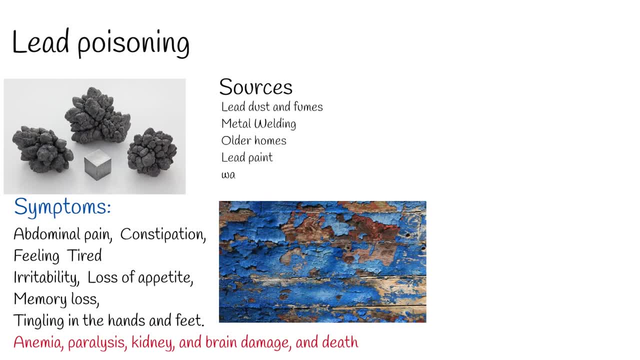 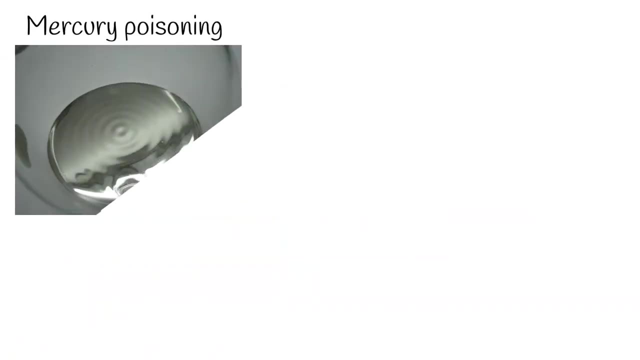 welding or working Older homes with lead paint and water pipes are major sources of lead intoxication. Other sources include firing ranges, battery manufacturing and cosmetics. Mercury poisoning. Mercury poisoning sources are sea products. also amalgam for dentists. a lamgam is filling material for cavities and in some countries it is still allowed. 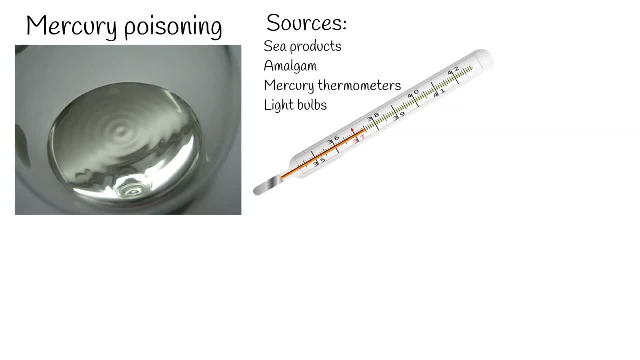 Mercury thermometers and mercury light bulbs also can cause intoxication if broken, Because mercury is hard to collect. If available, powdered sulfur may be applied to the spill in order to create a solid compound that is more easily removed from surfaces and liquid mercury. Mercury poisoning symptoms include 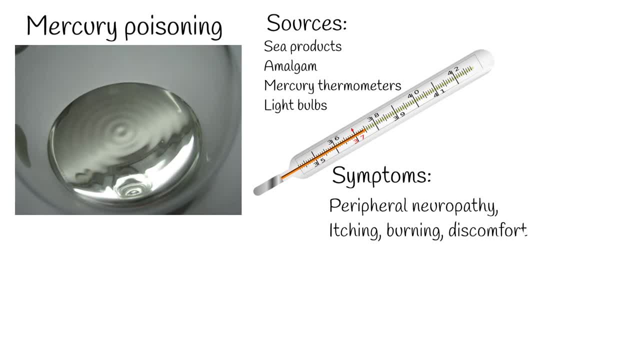 Peripheral neuropathy which manifests as paresthesia or itching, burning, discomfort or even a sensation resembling little insects crawling on or beneath the skin- formication. Other symptoms include profuse sweating, tachycardia, increased salivation. 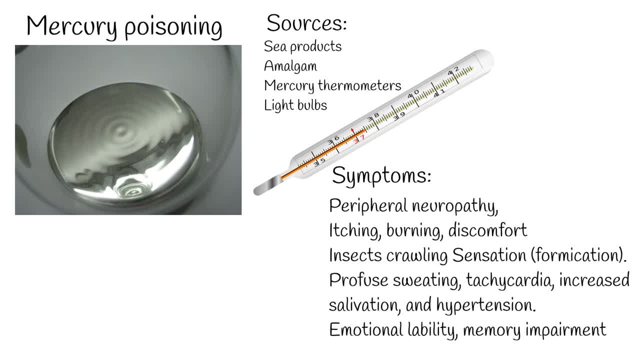 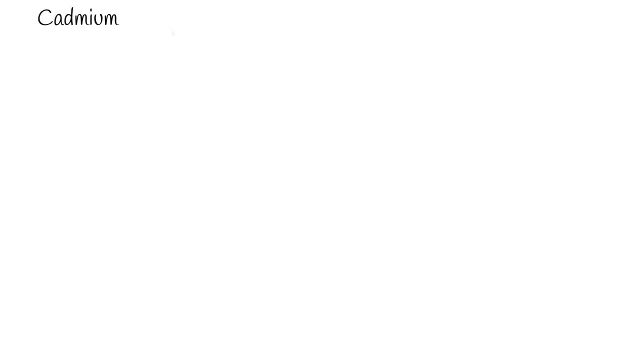 and hypertension. It can also cause psychiatric symptoms, emotional lability, memory impairment and insomnia. Most of mercury intoxication cases are reversible. it can have a much stronger effect on children. Cadmium Smoking is a significant source of cadmium. 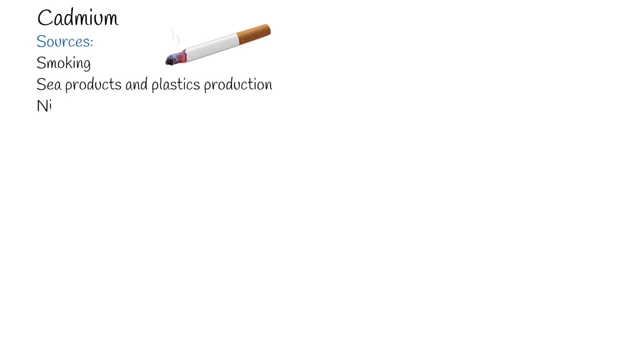 Other causes include sea products and plastics production and nickel-cadmium battery manufacturing. Acute exposure to cadmium fumes may cause flu-like symptoms. Heavy and chronic exposure to cadmium can cause complications of cadmium poisoning, including cough, anemia and kidney failure, possibly leading to death.